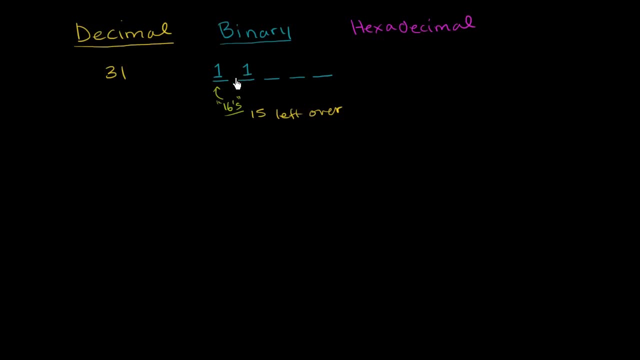 Let me just all do it in blue. So you have one 8.. And then, if you have one 8,, how much are you going to have left over of this 15?? You're going to have 7 left over. So then you're going to have 7 left over. 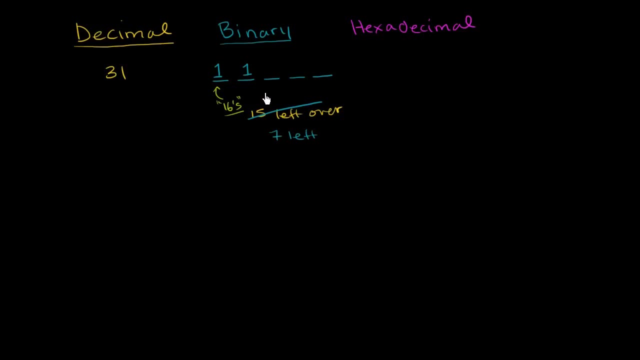 And so 8 doesn't go into it. Let's go to the 4's. You're going to have one 4.. And then, if you have that one 4, you now have 3 left over 3 left, And then we could take out one 2.. 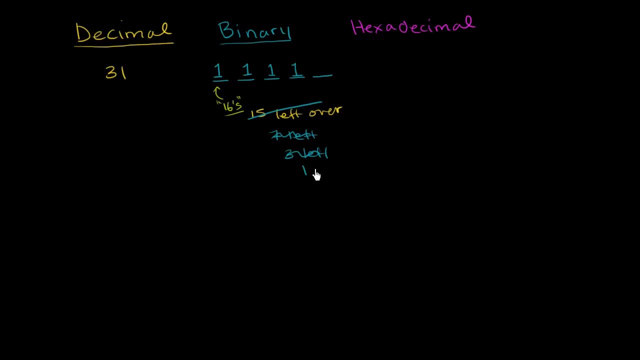 So then we'll have one left, We'll have one left And that 1,. we can just represent it as 1 in the 1's place, So it's literally 1, 1, 1, 1, 1 in binary. 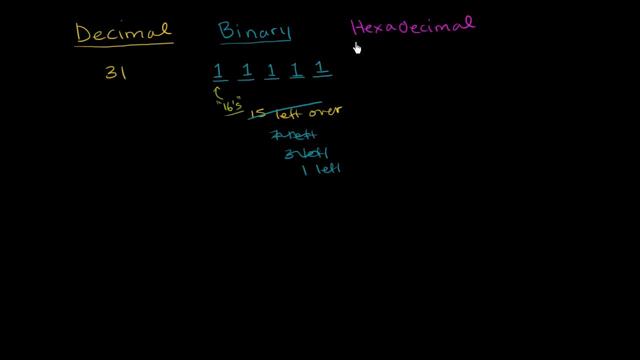 Now, in hexadecimal, what's the largest power of 16?? That is divisible into 31.. Well, just 16 is 256, isn't? So 16 goes into 31 one time. So let me make it clear: Here's our 16's place. 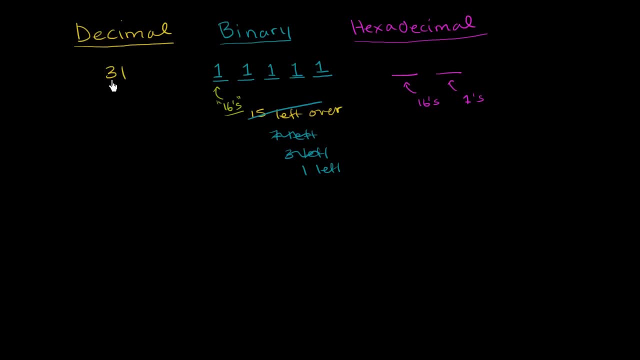 That's our 16's place. This is our 1's place. So 16 goes into 31 one time. So we have one 16.. And then you're going to have 15 left over, 15 left, 15 left over. 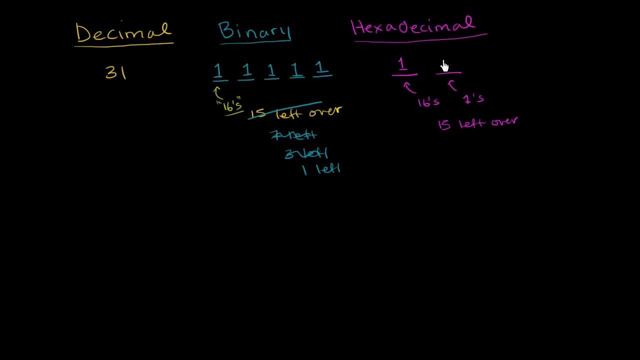 And you might say: wait, how do I represent 15 in one space over here? But remember, It's hexadecimal. Hexadecimal's have digits, have representations for numbers all the way up through 15.. Let me remind you, You can start at 0,, 1, you keep going. 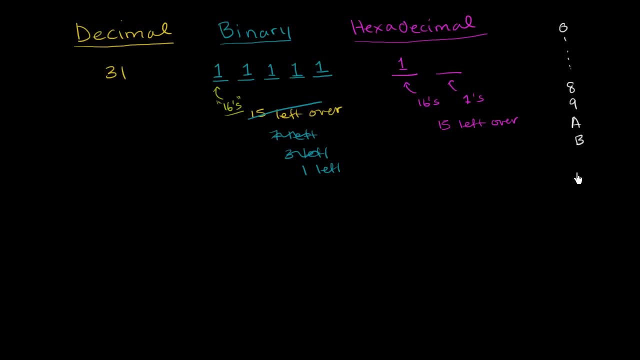 You go 8, 9.. Then for 10 you have A, For 11 you have B, For 12 you have C, D, E, F. F is the equivalent of 15.. So if you want to represent 15, 1's. 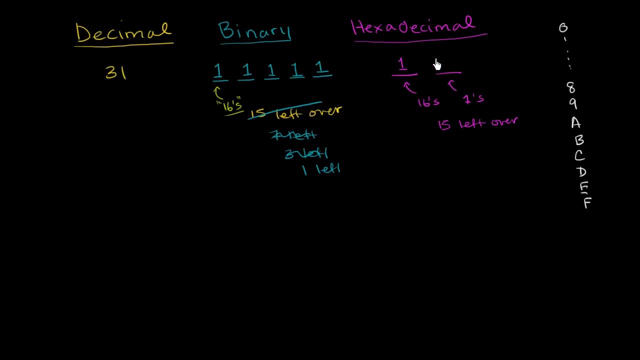 You literally just put an F here, So this might not look like 15.. It might not look like a number to you, But in hexadecimal it is 1F. This is hexadecimal for 31.. You have 1's 16.. 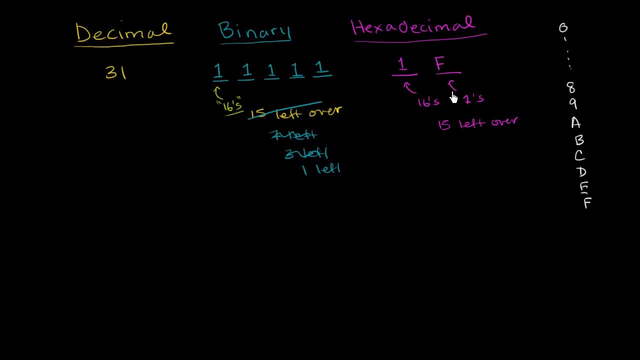 And you have 15 1's And this is the symbol for 15.. Let's do a couple of other examples And we'll convert between the different number systems. Let me think of a binary number. So let's say I just have 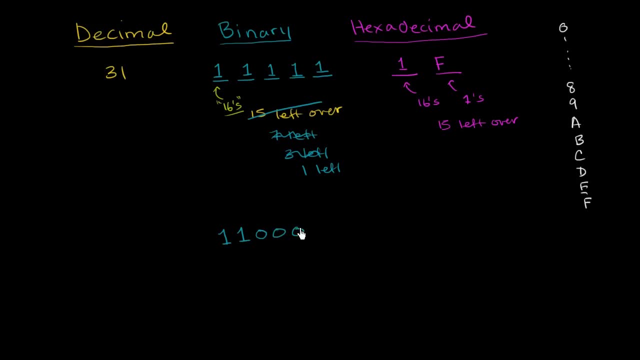 1, 1.. 0, 0, 0.. 0, 1, 1.. 0, 1, 1.. So this seems pretty complicated, But if we just break it down by the number spaces, 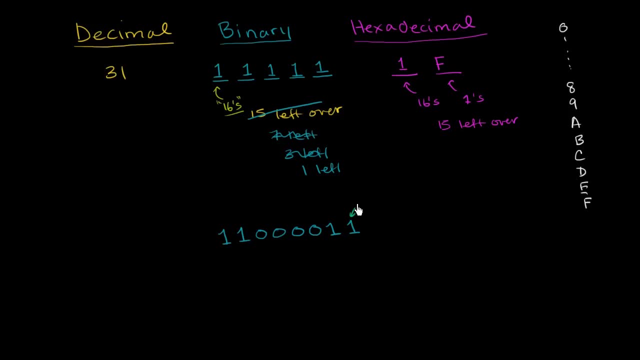 It shouldn't be too bad. So we have 1, 1.. So this is 1.. So you can just call that 1.. We have 1, 2.. This is the 2's place. now, Actually, let me write the places here. 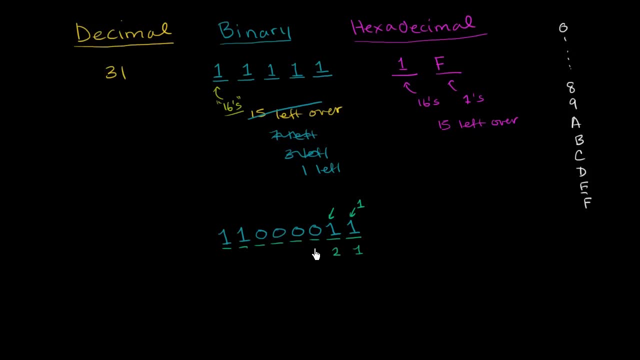 I think that will help clarify things when we're doing this conversion, Or at least as we start. This is the 1's place, The 2's place, The 4's place, 64. And then 128.. So you have 1, 1.. 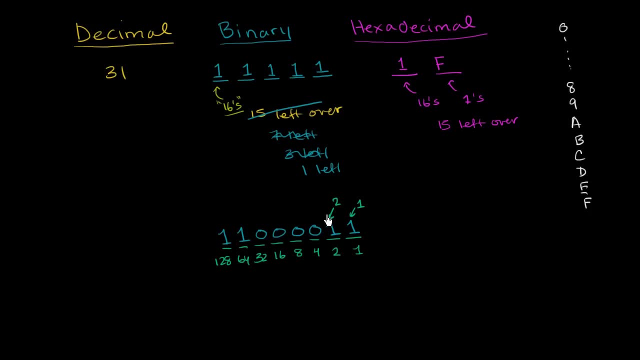 Which is just 1.. You have 1, 2. Which, if we wanted to represent it in base 2, we would write: Or larger base, Not base 2. In base 10. Or larger base than binary, You would call that. 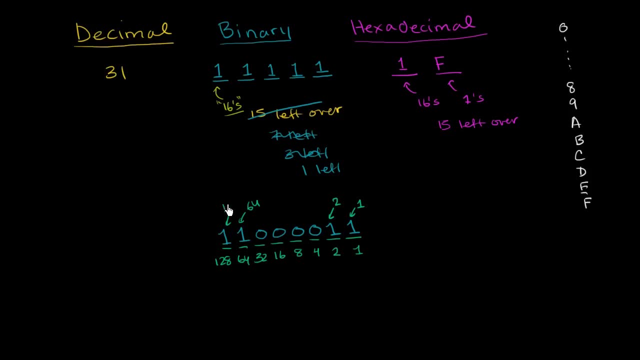 So that's 2. And you have 0,, 4.. 0, 8's, 0, 16's, 2 plus 1. So let me add that up. So if we have 128 plus 64.. 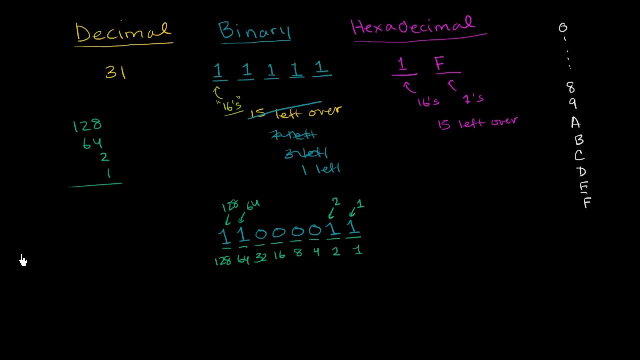 Plus 2 plus 1.. Plus 2 plus 1. You're going to have, You are going to have 8 plus 4 is 12.. Plus 2 is 14.. Plus 1 is 15.. 1 plus 2 is 3.. 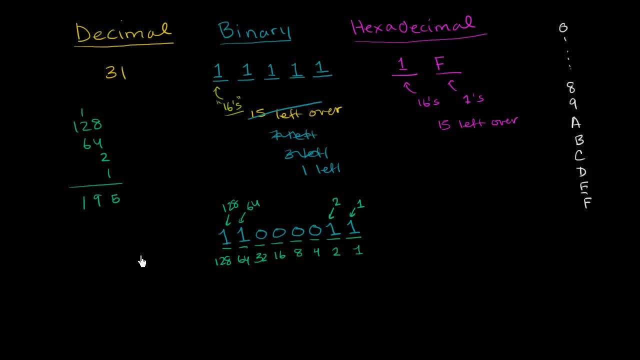 Plus 6 is 9.. And then you bring down the 1. So this: 1, 1. 0, 0, 0, 0, 1, 1.. In base 10.. In decimal, In a decimal number system. 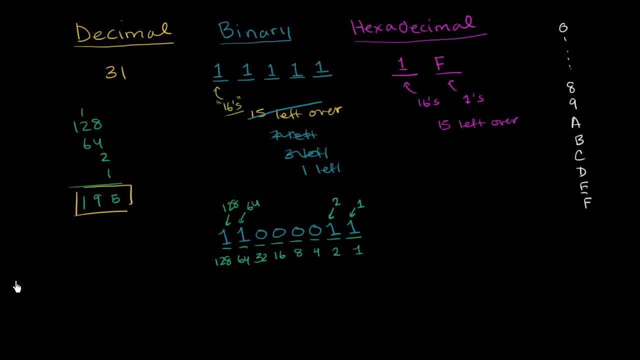 Is 195.. So how would we write this same number In base 16.. In base 16.. So the way to think about it, The way to think about it, Actually, there's a trick: to go straight from base 2.. 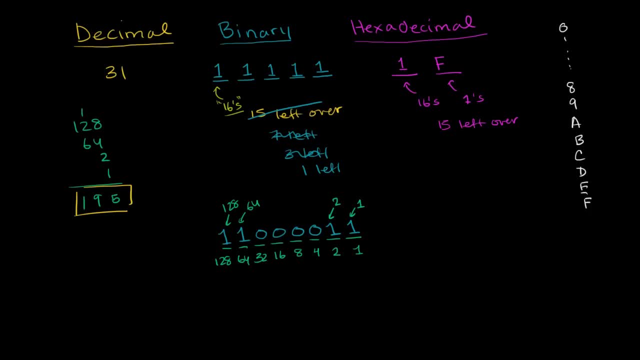 To base 16.. But I won't do that just yet. But the way to think about it is: Let's go. Let's say we have a 16 that goes into 195.. 256 doesn't go into it, So 16 is the largest power. 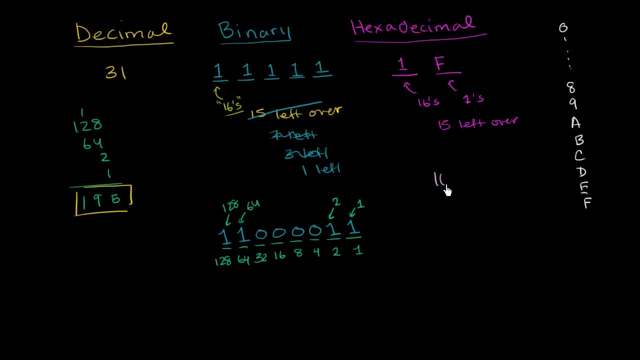 So how many times does 16 go into 195?? Let's just do the math: 16 goes into 195.. Goes into 19 once. 1 times 16 is 16.. Subtract, You get a 3. Bring down the 5.. 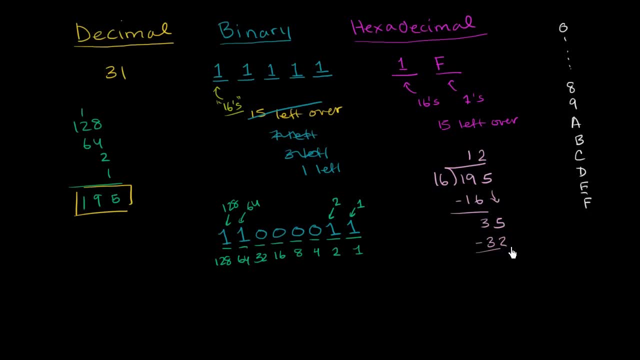 16 goes into 35. 2 times 2 times 16 is 32.. Then you subtract, You have a remainder of 3.. 16s plus 3 ones. So let me write it again: 195. you could write this as: 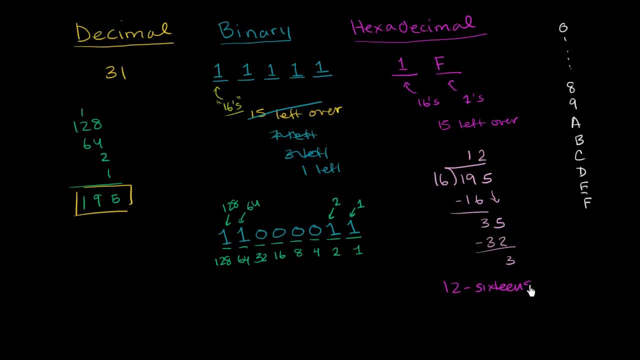 You could write this as 12 16s, 12 16s And then Plus 3 ones. Right, 16 goes into 195, 12 times. So you have 12- 16s And then you have 3 ones. 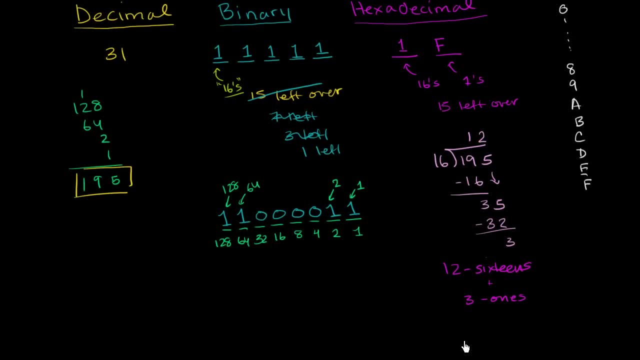 So in the 16s place. This might be a little bizarre, But the more practice we get will actually make a lot of sense In the 16s place, 12.. But we're going to write 12 using our new digits. 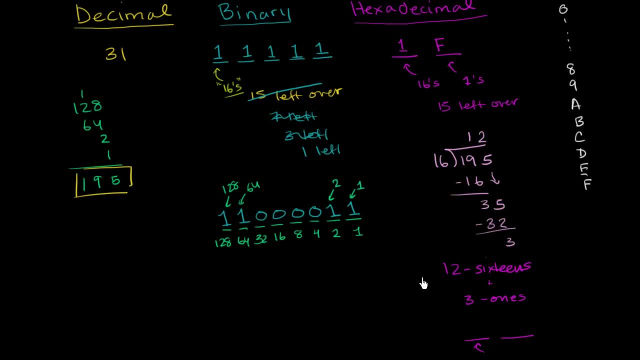 We don't want to write base, We want a symbol for it. We don't want to use our base 10 symbols right over here. So let's remind ourselves: A corresponds to 10 in base 10.. B corresponds to 1: 1 in base 10.. 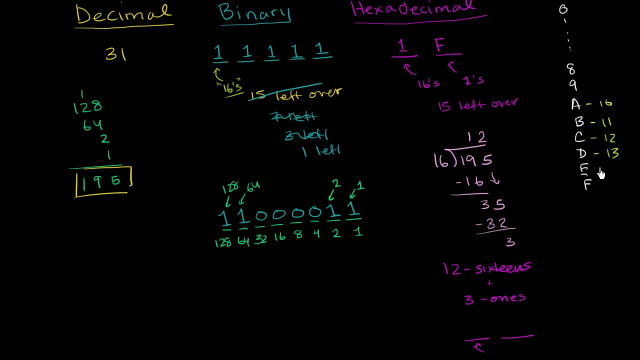 Or 11. C is 12. D is 13.. E is 14. F is 15. So to represent 12 in base 16. You use C 3 ones, So once again This looks more like a gate at an airport. 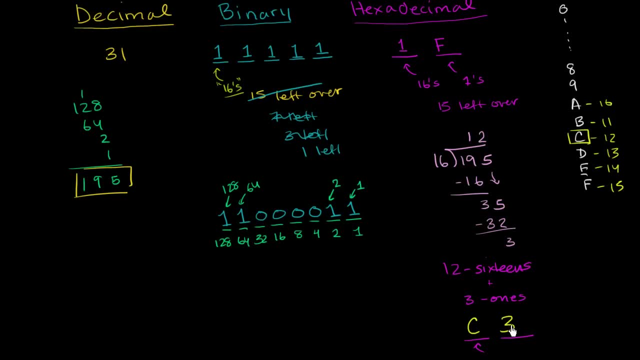 But this is actually a number in base 16.. C3. This is telling you you have 12.. This is a symbol for 12 in base 16.. You have 12 16s Because this is the 16s place. 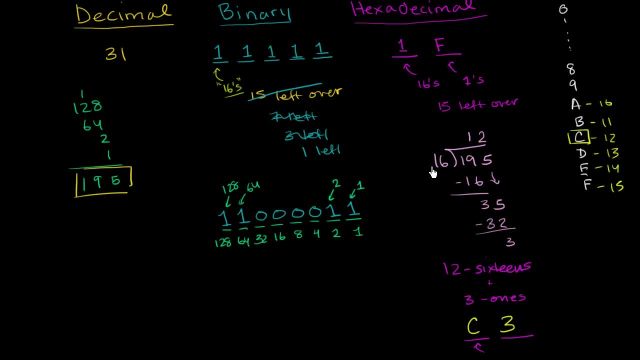 And you have 3 ones, 12, 16s. If you multiply 12 times 16. You get to 192.. You add 3.. You get to 195..